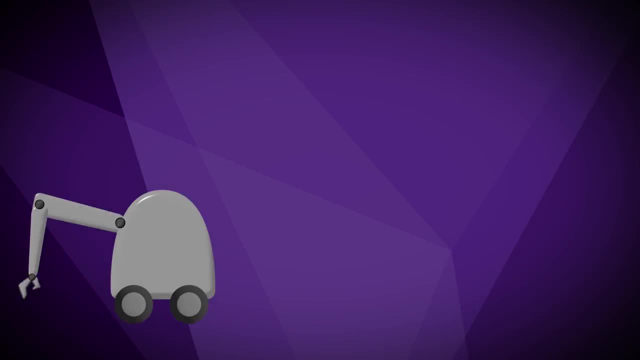 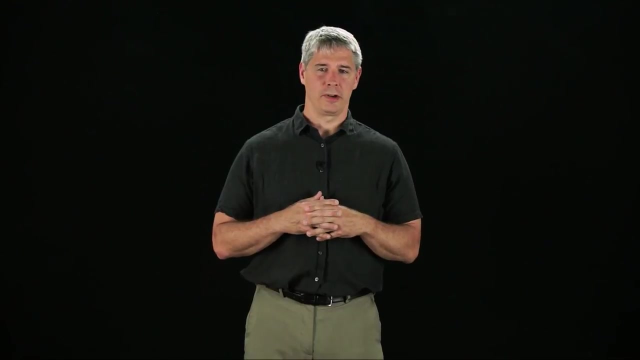 In the last two videos, we learned how to define straight line paths and then timescale them to get trajectories. If we want more flexibility to design the shape of the path as well as the speed with which it is executed, we could specify a set of configurations through 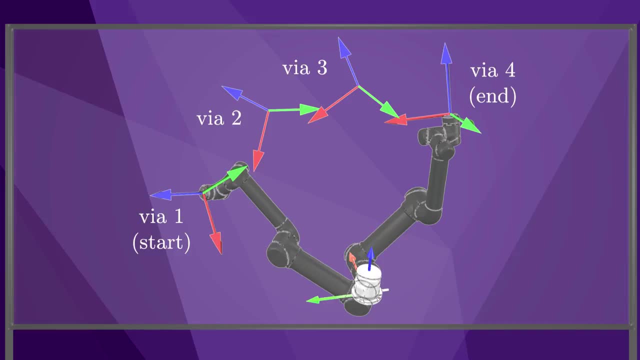 which we would like the robot to transit. These configurations are called via points. We also specify the times at which the robot should achieve each of these via points. We then solve for a smooth trajectory that passes through the via points at the specified times. 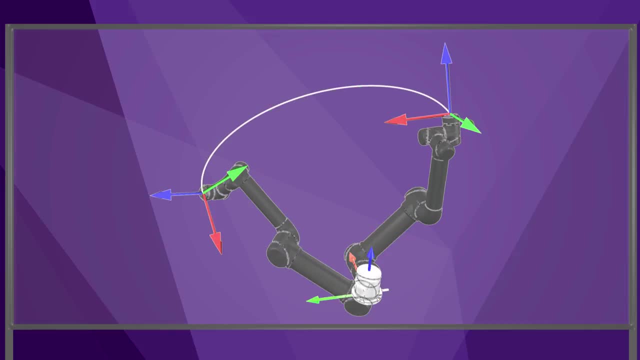 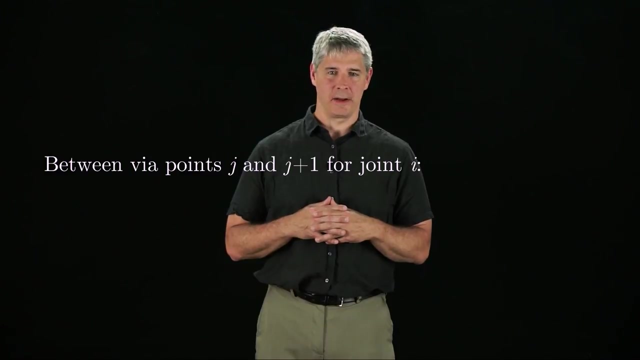 The choice of the via, points and times allows us to shape the path and trajectory. In this case we solve directly. for a trajectory, We do not first find a path and then timescale it. Let's consider motion in an n-dimensional joint space. For joint I, moving between via points J and J plus 1, we could define the. 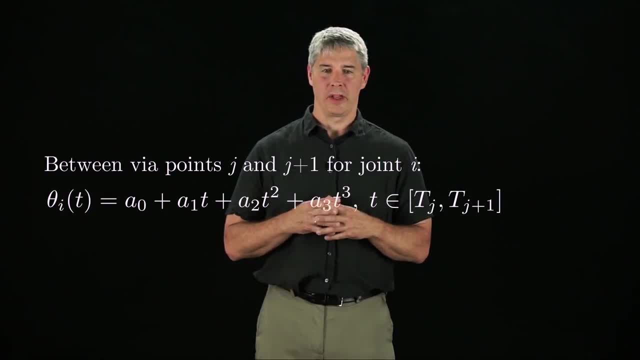 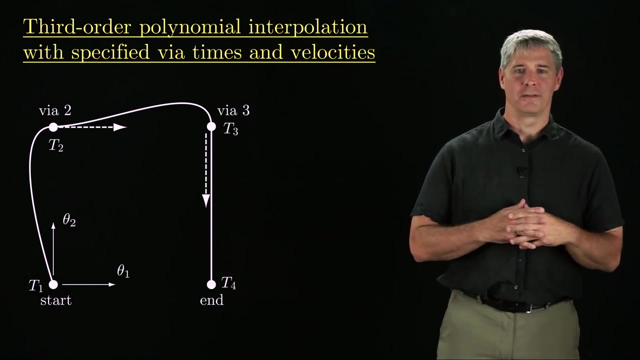 motion as a third-order polynomial of time. We then apply four terminal constraints, the initial and final position and the initial and final velocity of joint I to solve for the four coefficients of the polynomial. This is third-order polynomial interpolation with specified via times and velocities. This figure shows a path designed for a two-joint robot. 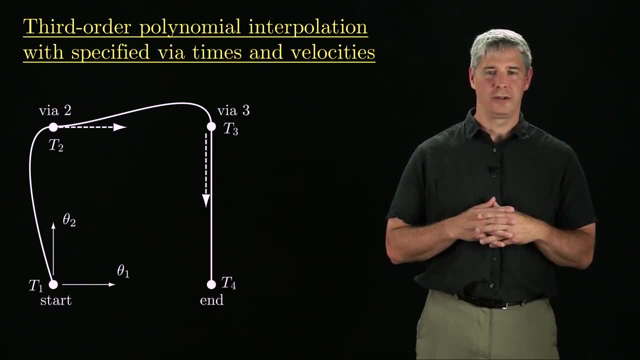 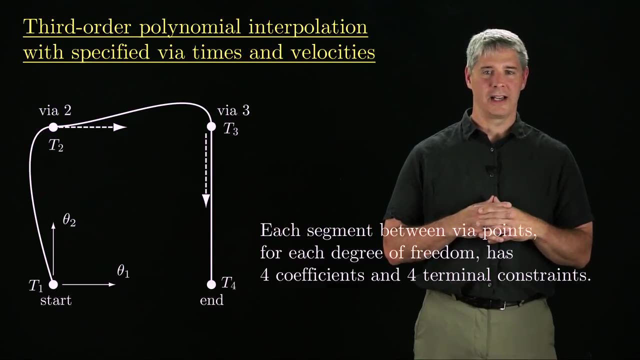 using four via points: the start point, the end point and two other vias. Each via point has the time that the robot passes through the configuration as well as the velocity at that time. The velocity is indicated by the dashed arrows. Each segment between via points, for each degree of freedom, has four coefficients. 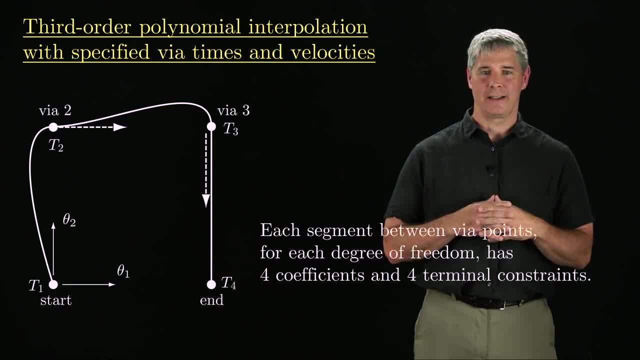 and four terminal constraints, which allows us to solve exactly for the trajectories between via points. The tangent of the path has to be aligned with the specified velocity at each via point, so we can use the velocities at the via points to change the shape of the. 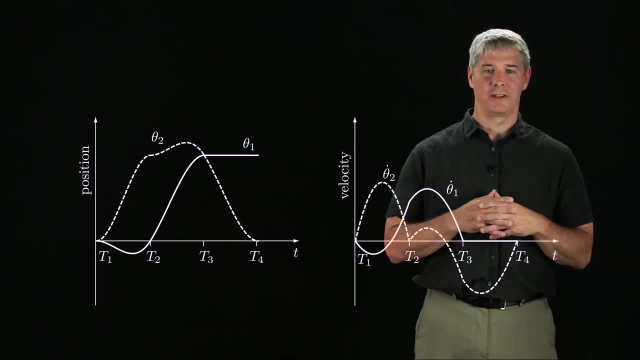 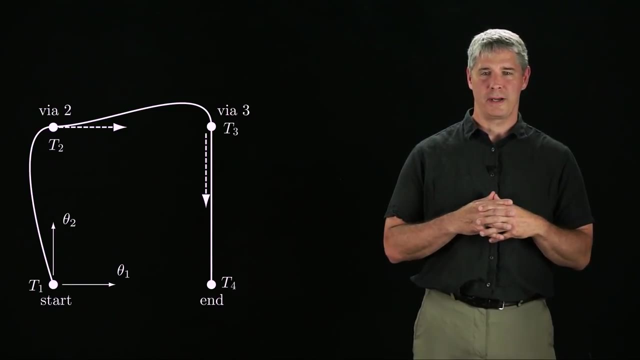 path. These time plots show the position and velocity during the trajectory. You can see that the positions and velocities are continuous at the via points, but the acceleration is not. Discontinuity in the acceleration may not be desirable. Also, it may be cumbersome to have to specify the velocity at each via point.